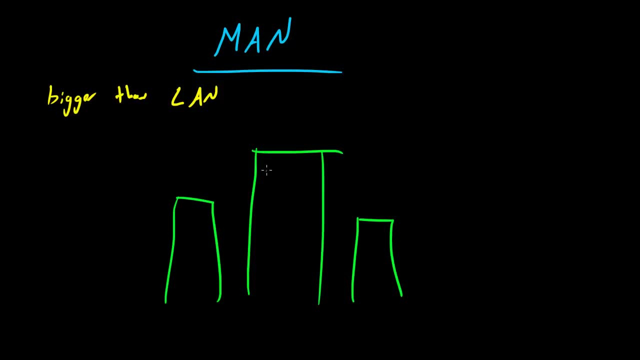 often span large cities. So you know, if you live in a big city, all of the computers connected in the city- and this, by the way, is a city- all of these computers could be connected. These blue things are computers, by the way. Computer in this building. 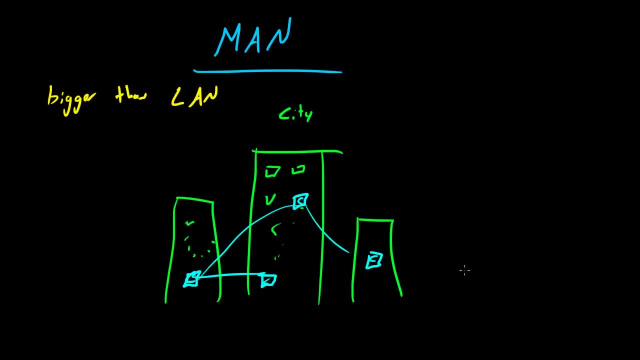 computer in this building. all across the city, different buildings and, you know, different homes too, can have computers. Draw a computer in there connected. These would be a man, a metropolitan- I better write that down- metropolitan area network. So remember: A- it's bigger than the LAN and B- it spans large cities. 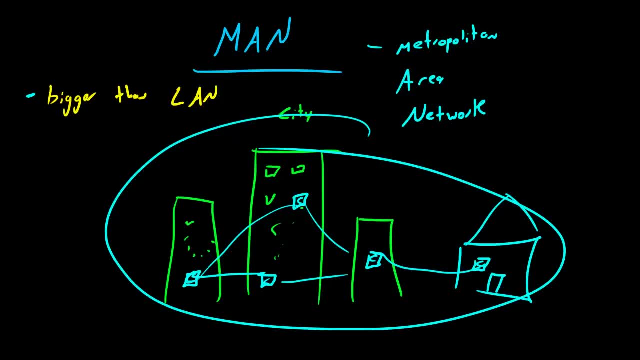 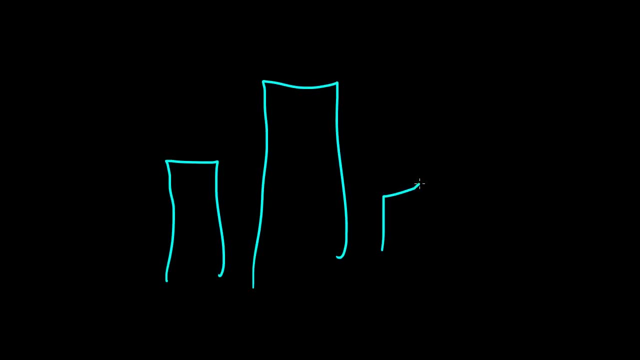 or maybe an entire grid. So you know, if you live in a big city, all of these computers could be connected. So why on earth would you want a man? Well, for example, it isn't that everyone in the city just decided to, you know, connect their computers. Say that you had a. 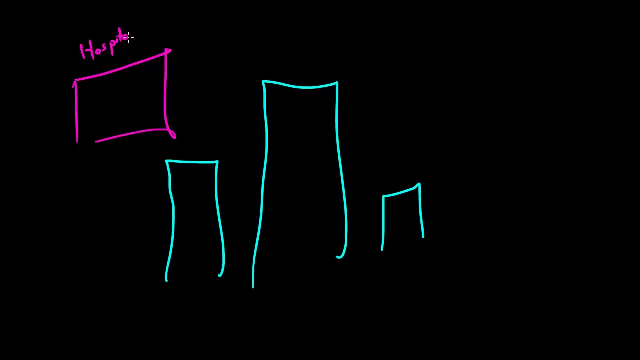 hospital on this side of the city and a hospital- I don't know, maybe it's a children's hospital- on this side of the city and way over here. I don't know, maybe you have some college or something like that, So you know if you live in a big city, all of these computers. would be connected. Now remember, if you live in a big city, all of these computers would be connected. So you know if you live in a big city or something like that. So you know if you live in a big city or something like that. So you know, maybe you have some college doing. 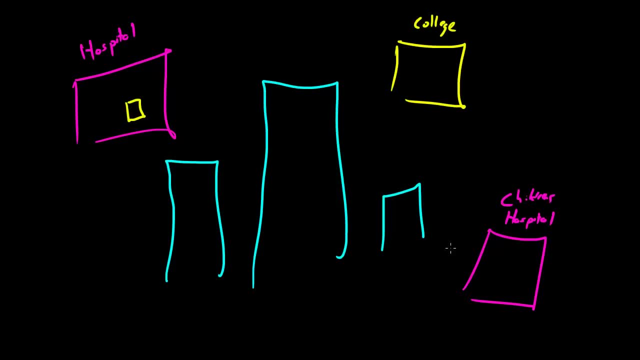 research. Well, these hospitals would want to communicate with this college. So what it would do is it would form a huge computer network, But since they aren't in the same building, what they would need to do is they would need to span this computer network across a very big distance. 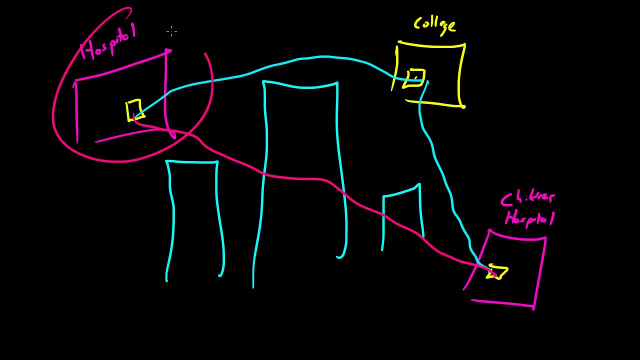 perhaps the size of the entire city. So this computer network, made up of a few hospitals and perhaps a college or two, could form a computer network and interconnect their computers so they can, you know, share research. or maybe the hospitals might just want to share patient information. 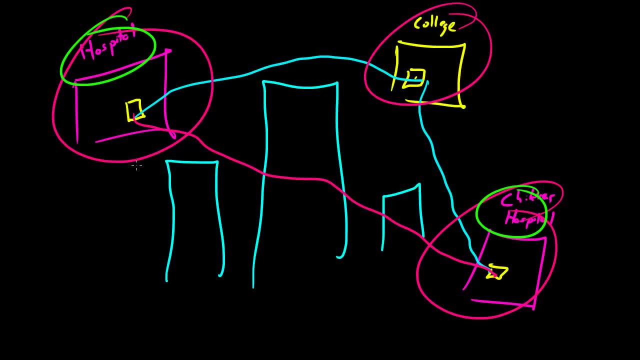 But basically, whenever you have a computer network which is just a bunch of computers connected to one another and it spans an entire city or, you know, maybe a county- this would be a man Metropolitan Area Network And the types of media that they use to transfer data- again, it used to be cable.